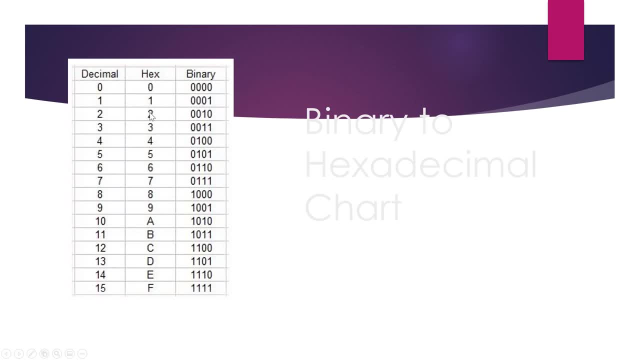 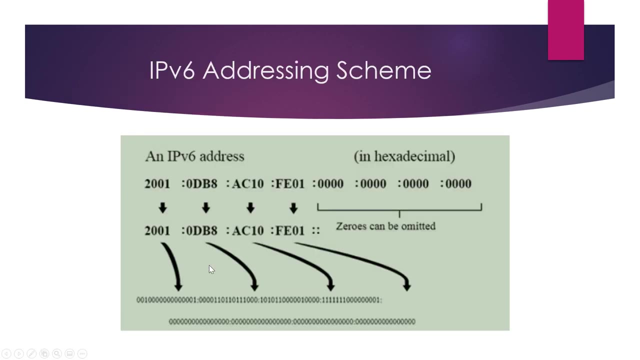 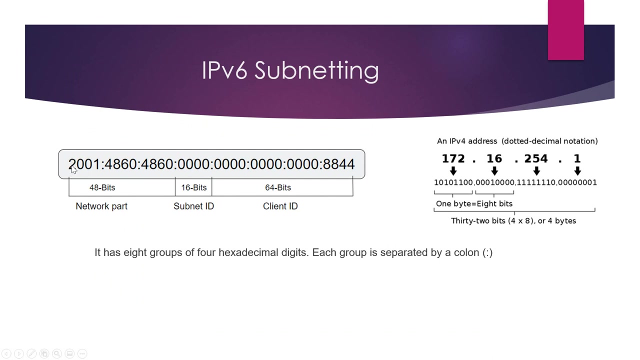 And each hexadecimal digit- this is a hexadecimal digit and it is the equivalent of decimal digits- And each hexadecimal digit is represented by four bits. So that is how you get 16 bits. So each is four, And so So you multiply four into four, you get 16-bit, and you add the 16 into eight, that come up to 128 bits. 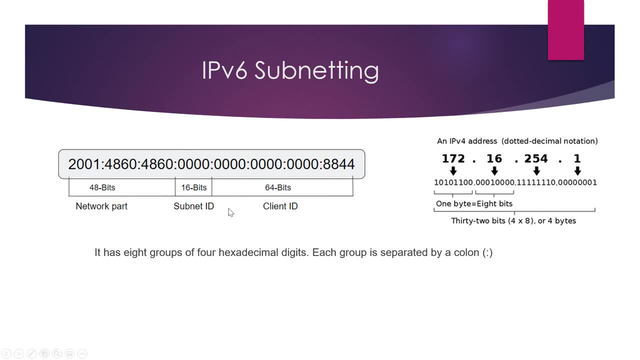 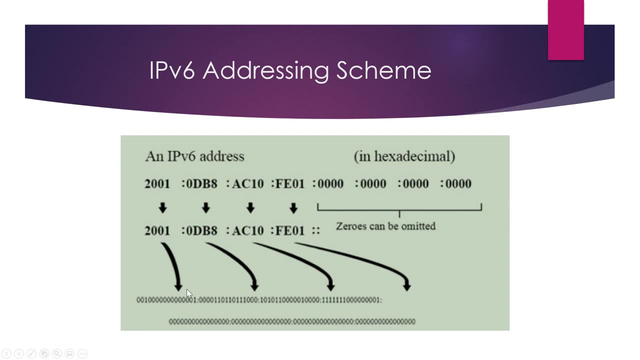 And out of this, this is the subnet ID, But it is not always the subnet ID. You can have this also as a subnet ID. So let me explain to you when I do the calculation. This slide is about you know how you come up with this hexadecimal digits. 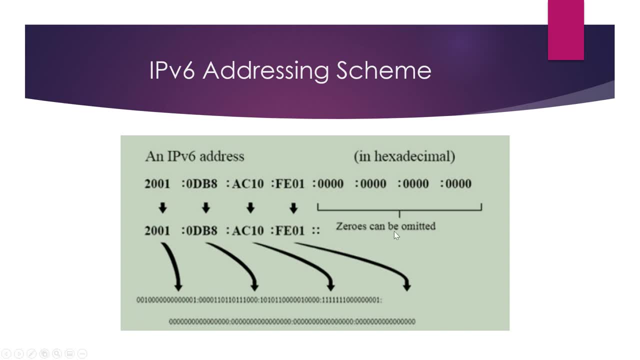 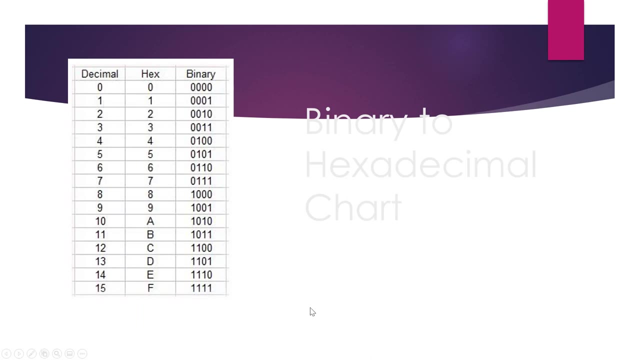 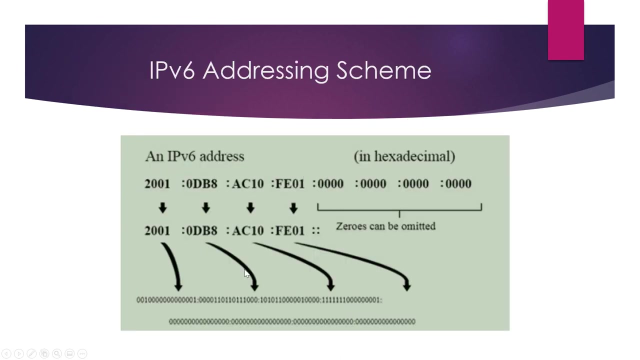 Like a two is that 0010, and if you go here, two is 0010. And so everything else is zero and one is 0001, and one is 0001.. So you need to use the chart to figure out what is this number is going to be. 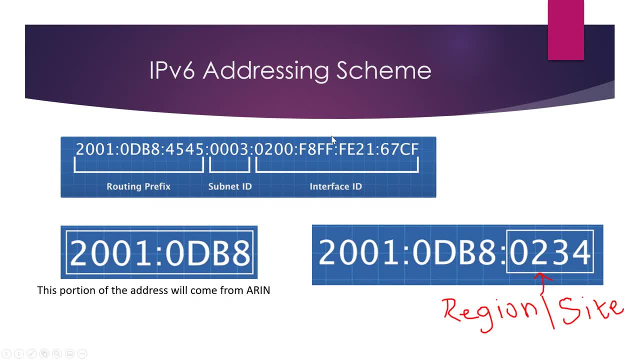 So let me come to the next one. So let me come to the IPv6 addressing scheme. So this is the routing prefix. In the routing prefix, these two numbers come from ARIN, That is your internet registry. It depends on where you live, and there are five of them worldwide. 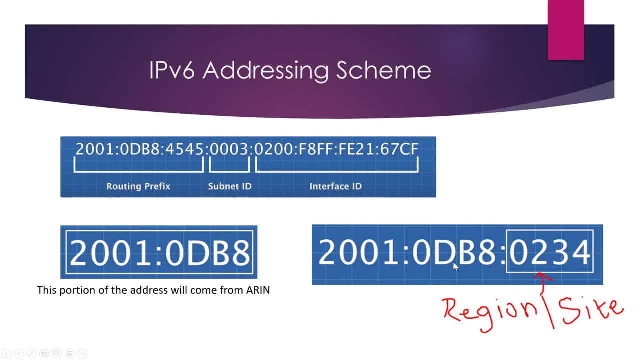 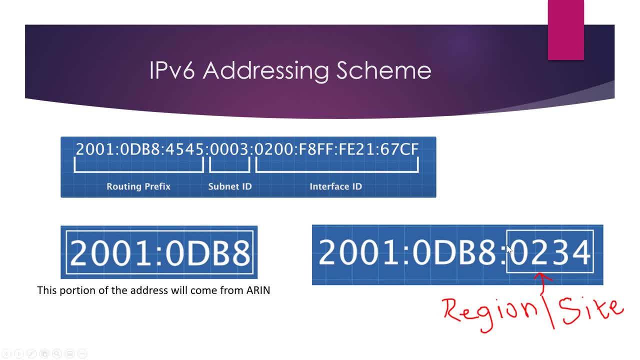 So if you are a university, you can decide, you can change this number because you are a region or you are a site And this is all allocated for host. So out of this 128 bits, 64 is strictly allocated for host. 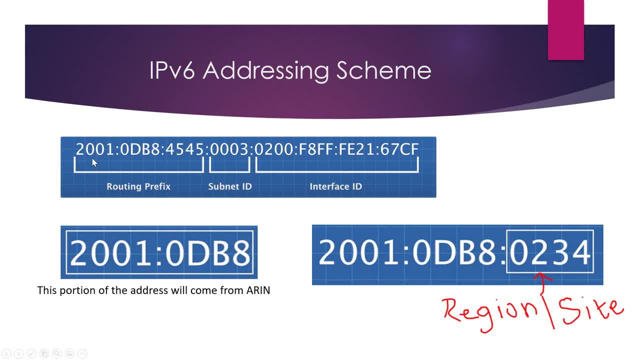 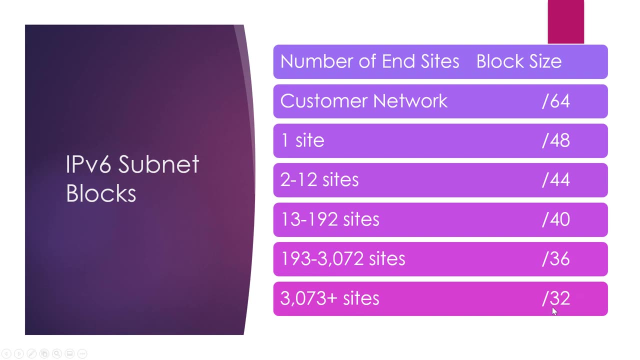 and the rest of 64 is for routing and subnet purpose. So this is what we are going to use for our subnetting. So if you are a large site, very large site, you will be provided with a 32-bit address, That is say, if you are an internal service provider or a big 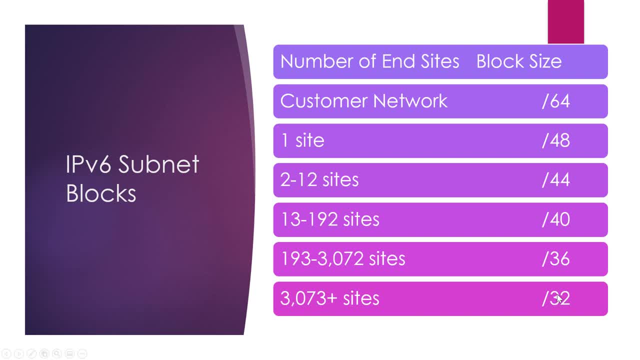 large university, you will be provided 32.. And then, if you are a small organization other than these, it can be 36 or 40,, 44,, 45. This is an internal service provider. You don't need an application. 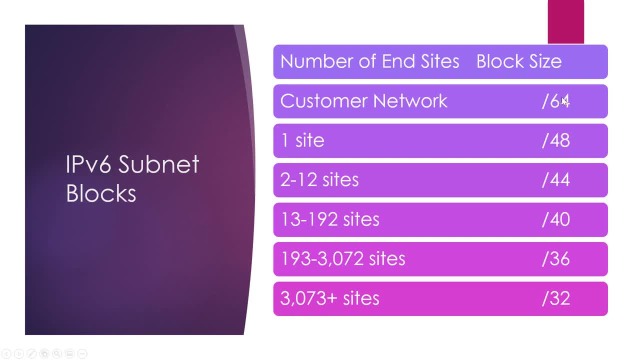 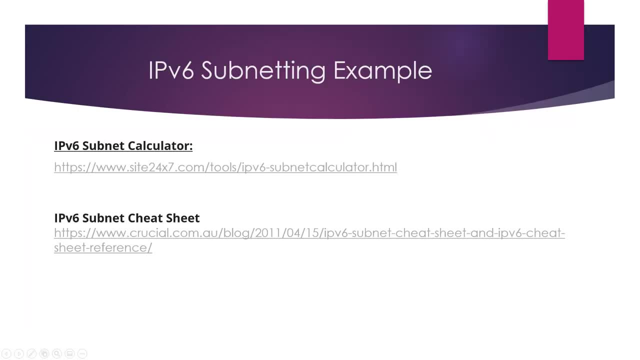 48. 64 is the customer block. so if you have a subnet called 64, that is called a customer network. so i'm going to use a calculator here. this is the subnet calculator, so let me bring it here and also i am going to use uh, this one. this is a cheat sheet for ip version. 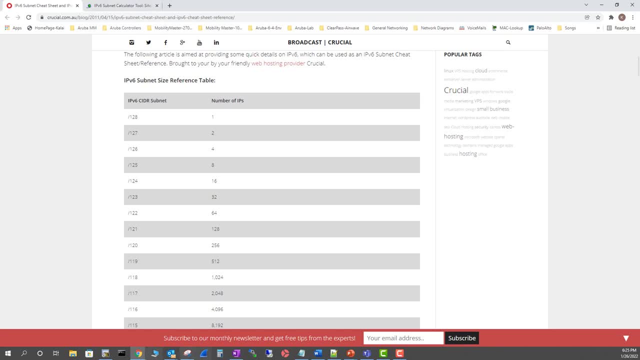 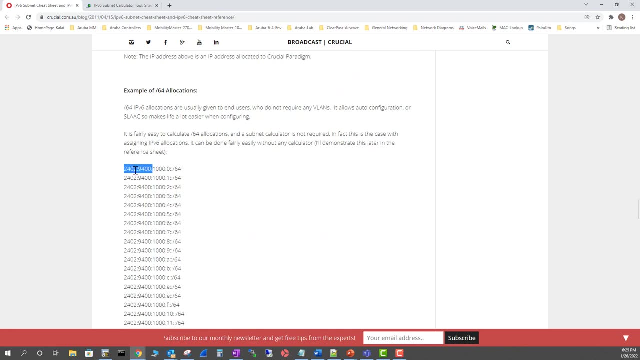 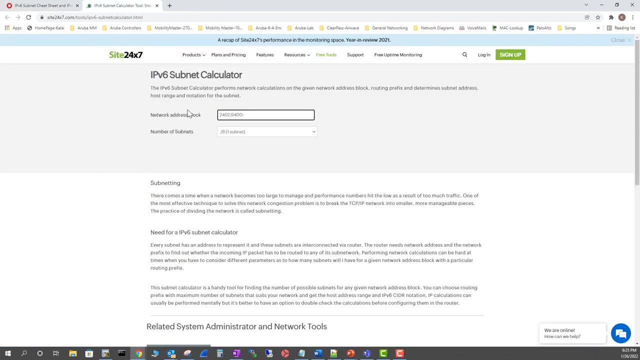 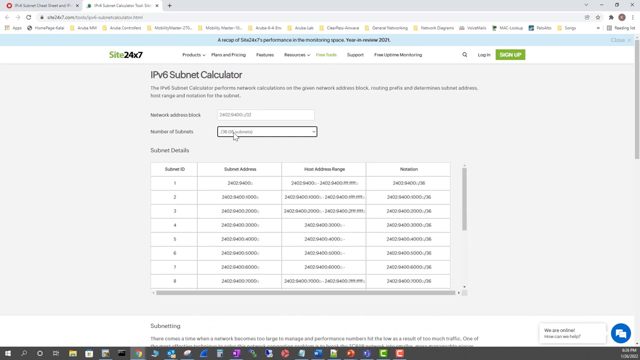 uh six. let me show you how to do the subnetting. so i'm going to grab a address here, a real address. think about you get this one uh slash 32 for your university. so you go here and this is going to be uh 32, and the best practice is you take this 32 and slide this up into 36 so you will get 16. 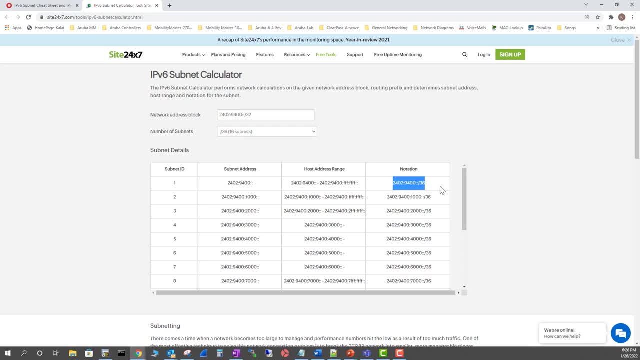 36 subnets and you take the, the first one, and you divide this. you divide this into another 60, that is going to be slash 40. and you take one of that slash 40 and divide that up into another 16, that is 44.. 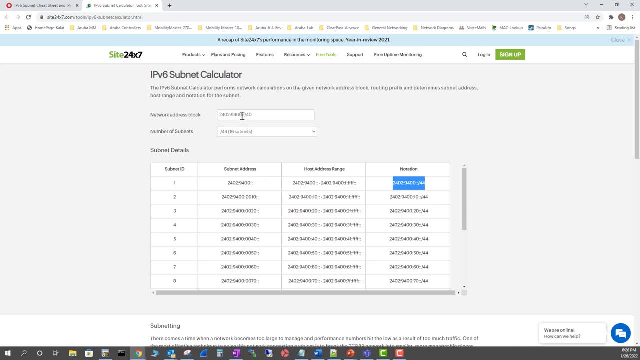 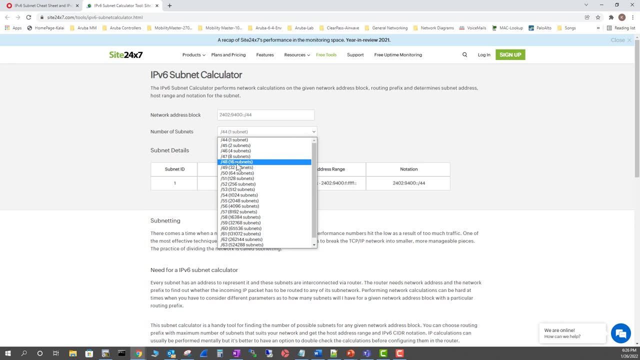 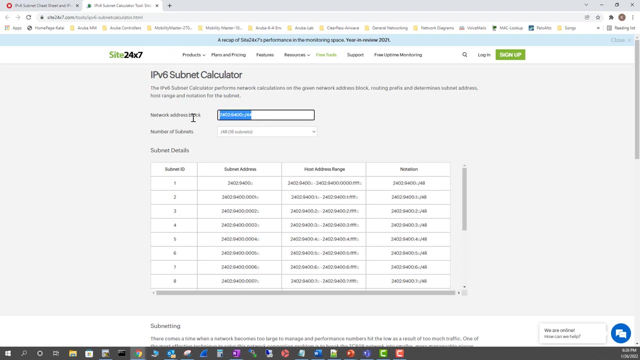 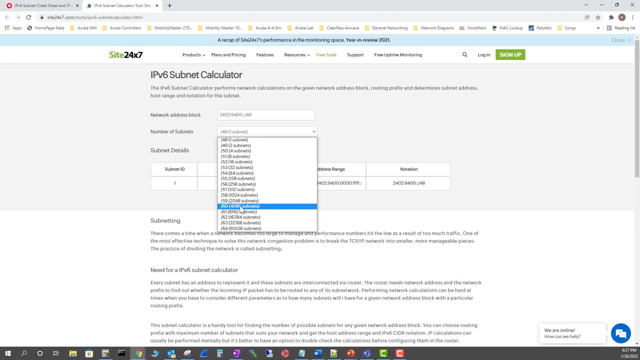 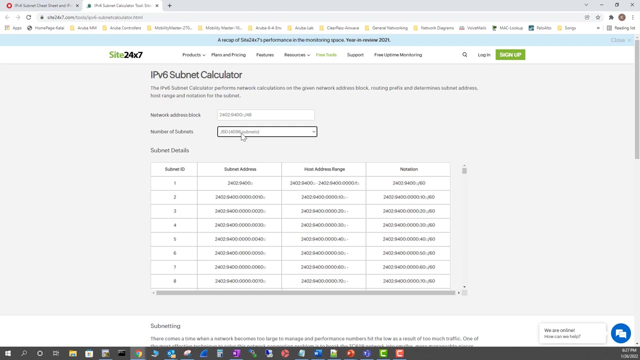 and you take one of this and put it here and then divide this up into 16- 48 subnet. and you take one of this and put it here and then divide this into whatever you wanted. so you can have a 60 um subnet and you will have 4096 slash 60 subnet. and if you take 160 here, 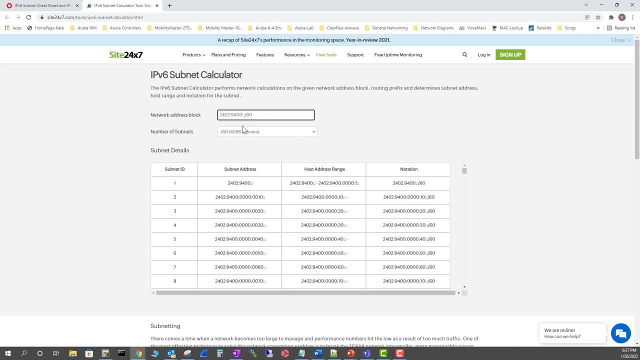 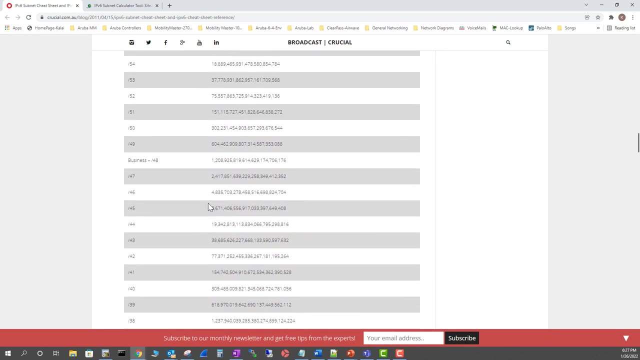 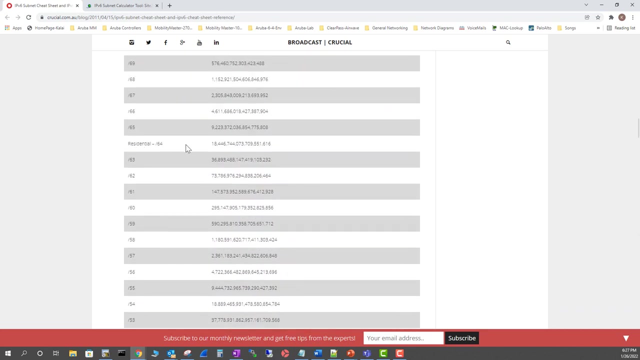 and put it here, and then you can have 16 slash 64, which is the customer subnet, and if you go here and find out how many hosts you can have in slash 64, it will be mind-boggling. and if you go here, this is the customer residential network- you can have this many addresses. 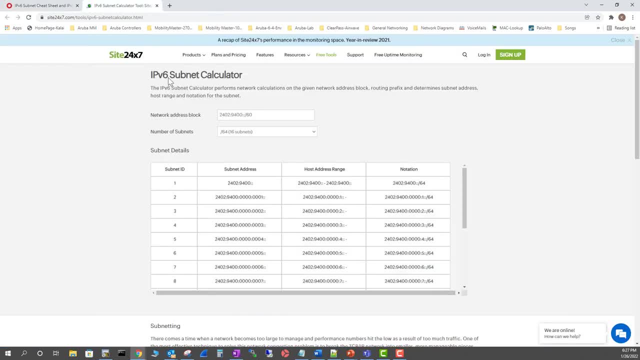 in this subnet and you can have this many addresses in this subnet and you can have in just one single 64, and you know how many times i have divided this 32 into multiple subnet. i think i must have divided so many times and you now know how many addresses you can get. 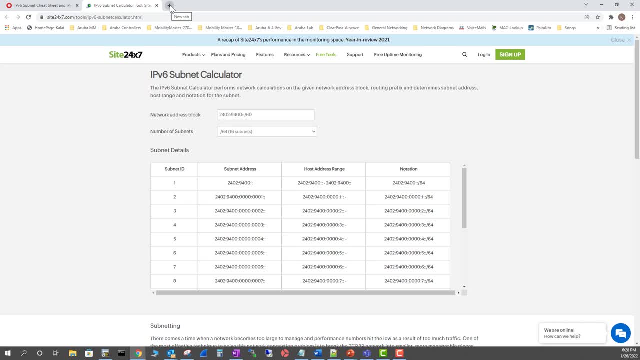 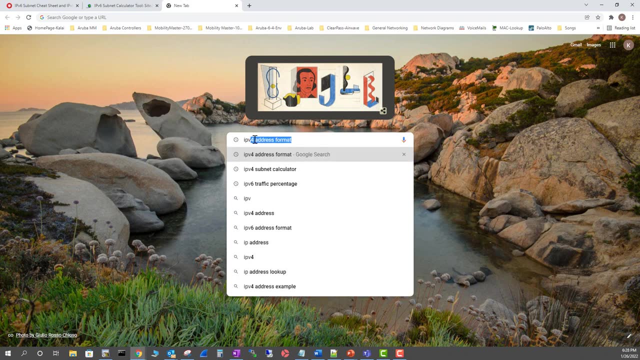 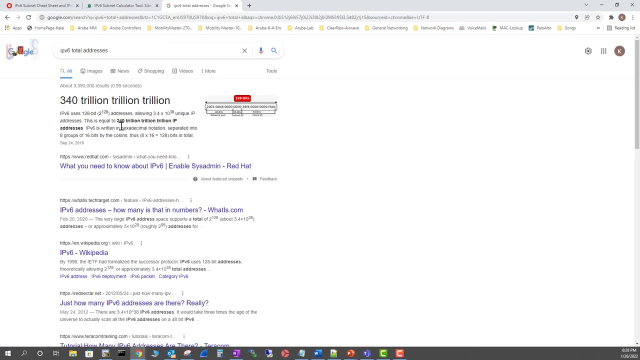 in ip version 6 networks. so let me show you how many address you can have in ip version 6. that's ip version 6 and you can have this many addresses in this subnet and you can have ip version 6 total address and if you see, here you can have 340 trillion, trillion, trillion. so you 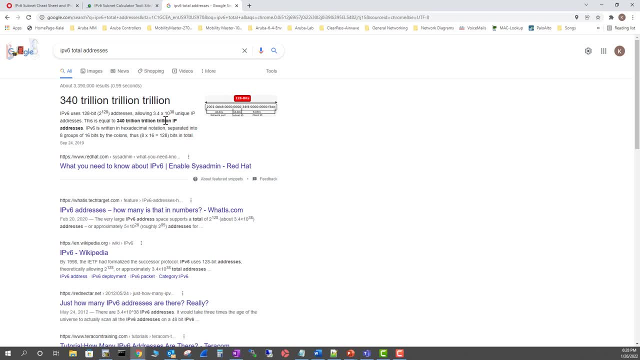 multiply 340 into 3 trillion- that many ips you can have. so the concept here is you never going to get an ip depletion with ip version 6.. i hope you like this video. if you like, please hit the like button and subscribe to the channel. if you want to more video. 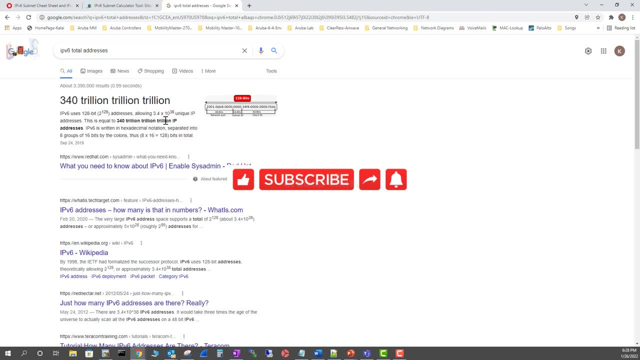 from my channel. just turn on the notification. uh, okay, thanks so much. i will see you next time. bye.